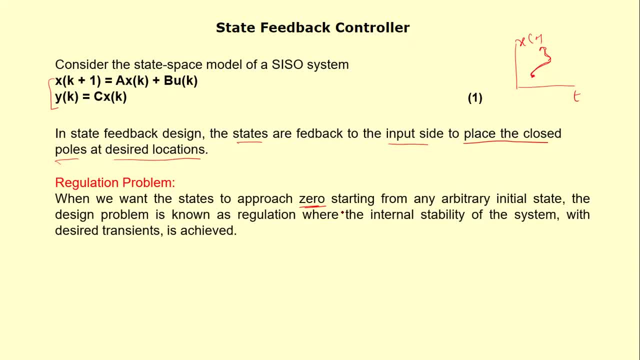 some equilibrium point. so this problem is known as regulation problem, where we actually study the internal stability of the system. that is, the regulation problem is- uh, you know, is associated with the internal stability of the system, and by bringing the state of the system from any arbitrary initial state to zero, we actually are achieving the internal stability of the system. 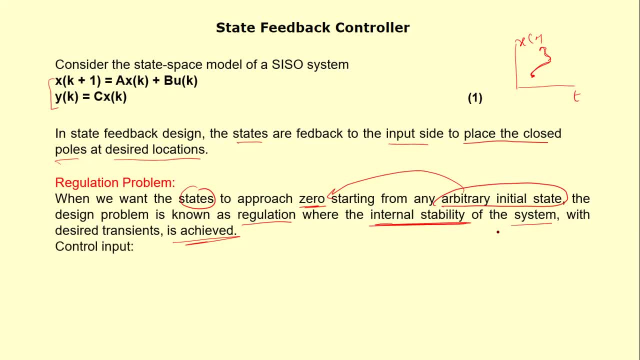 right then. second problem now. in this the control law that is used is u k minus k into x k, so this equation is called the regulation problem. equation number two: now then we have tracking problem. now, in tracking problem, uh, the output, the response of the system is tracked. uh, in reference to the 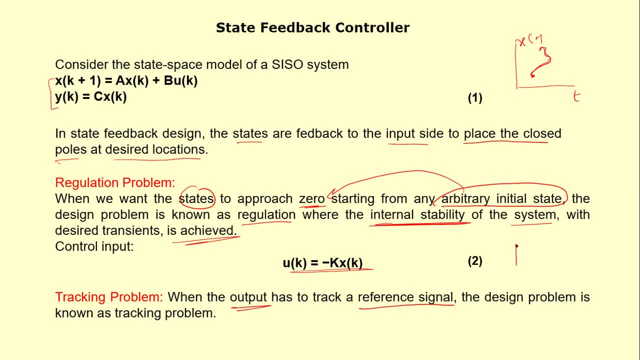 reference signal: right with respect to the reference signal, okay, so if the reference signal is uh, you know, let us say uh, like it is a step, uh input, so the output, uh is tracked, okay, signal is changing with time, so the response is: you know, should also change, right, so this problem. 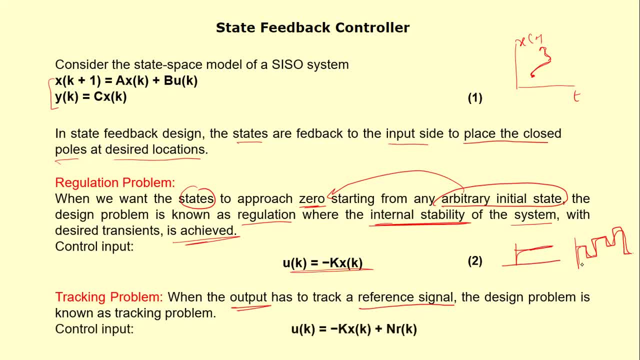 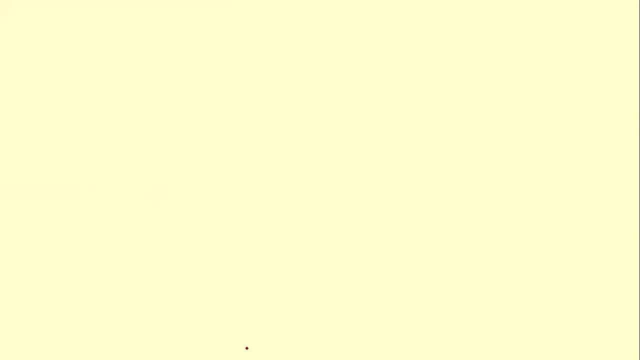 is known as the tracking problem, and the control law, the control algorithm that that is used for this problem is given by this equation, where rk. here is the reference signal now. now, first of all, we will discuss the state feedback controller design using pole placement technique for regulation problem right. 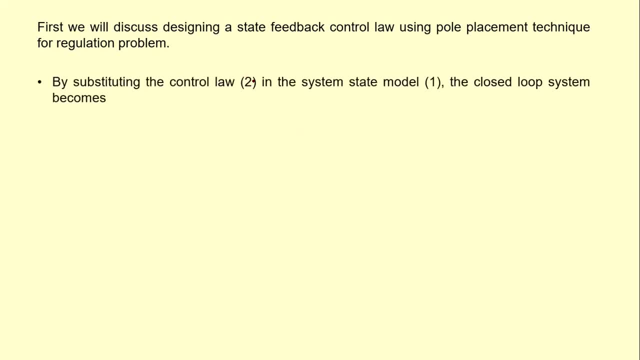 so if we substitute the control law that is given by equation 2- and the control law given by equation 2 is uk is equal to minus kxk and if we put this in equation number one, that is x k plus 1, is equal to a, x k plus b. u k right. So if we substitute this u k, 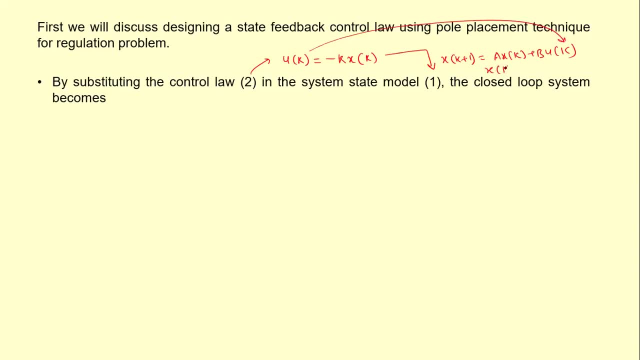 here. So we will get: x k plus 1 is equal to a x k minus b k x k, right? So this will give us this equation here, right, Okay? So now we can design this case such that the eigen values of 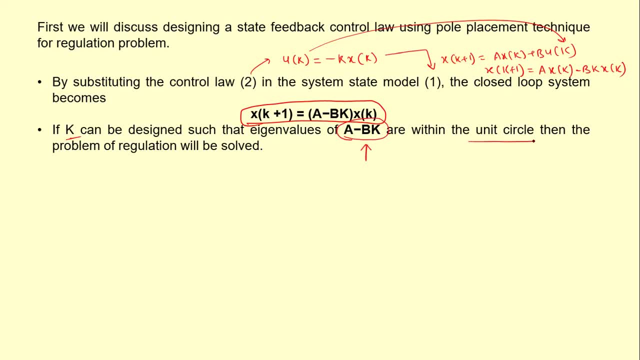 this matrix right. they lie within the unit circle because we are dealing with the discrete systems. So we do the stability analysis of a discrete system in z domain and we want that the- you know- closed loop poles of the given system should be located within the unit. 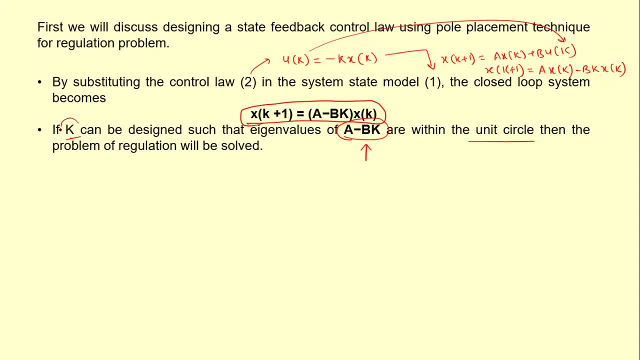 circle right. so if this k, if this k can make the eigenvalues of this closed loop equation to place in the within the unit circle, we can say that the problem of regulation is solved. this means that we will be able to bring the states of this system from any arbitrary- uh, you know- value. 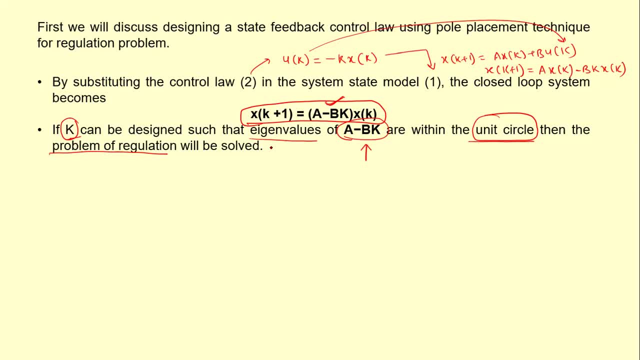 or initial state to the zero right. so, uh, we can define the control problem for state feedback controller as that you know. you know we have to design a state feedback gain matrix k such that the control law given by uk is equal to minus kxk can place the poles of the closed loop system. this in the desired locations, right? so this? 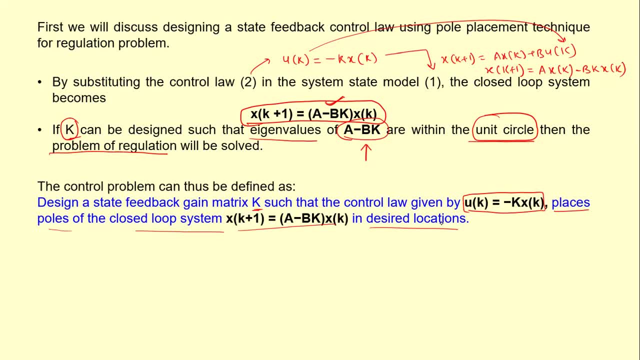 is the- uh, you know- statement or control problem that we have defined and we would be working on, uh, you know, this control problem and our purpose is to obtain the state feedback gain, matrix k. now there is a necessity and sufficient condition for this, and the necessity and sufficient condition for this is that, uh, the 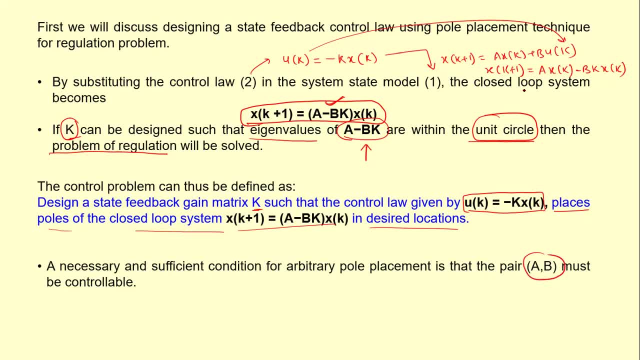 pair ab. so here ab is from the state equation, right, okay, so it must be controllable, right. and the second, no, uh, second thing is that because all these states of the system are sent are fed back to the input side, so we assume that all states are measurable. so if we see the block diagram of this, so this is a delay. 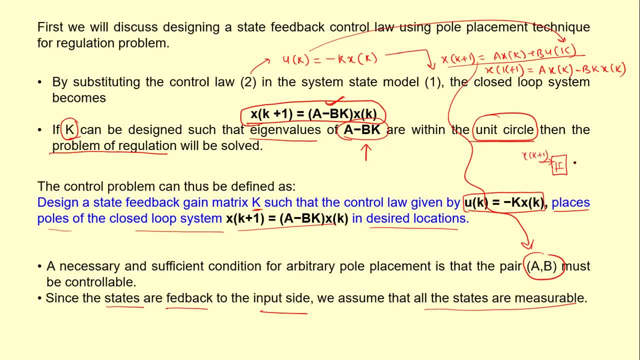 element. it has input xk plus one and the output here is xk. and we will feedback this xk, the state by multiplying this with some matrix a to the input side, right here we are adding this with- uh, you know, b matrix and the input is uk, right, so we can see that it is fed back to the 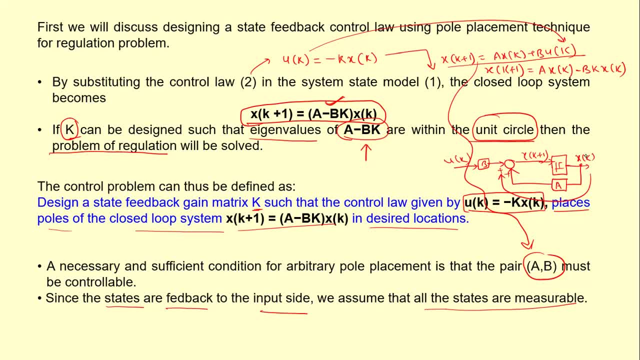 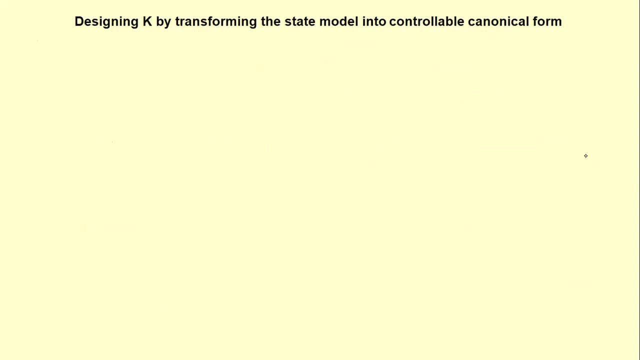 input side, the states are fed back to the input side, right? so if we are feeding these states back to the input size side, so it means we are assuming that all states are measuring and lying between the different states, you accordingly. so by doing this we can monitor. 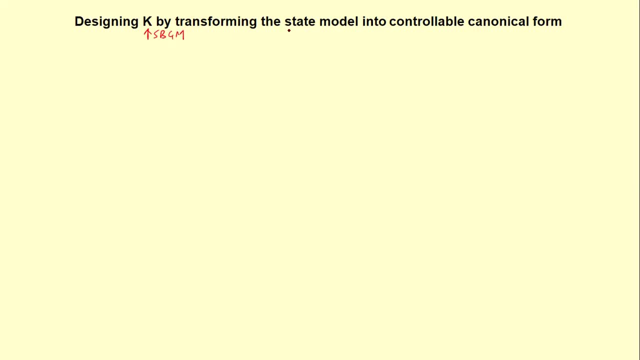 thisсти glucose level for every single state and the benefit we get is, so it allows perf, Unbelievable. now let us design k the state feedback gain matrix. this is state feedback gain matrix by transforming the state model into the controllable canonical form. the first of all because we want 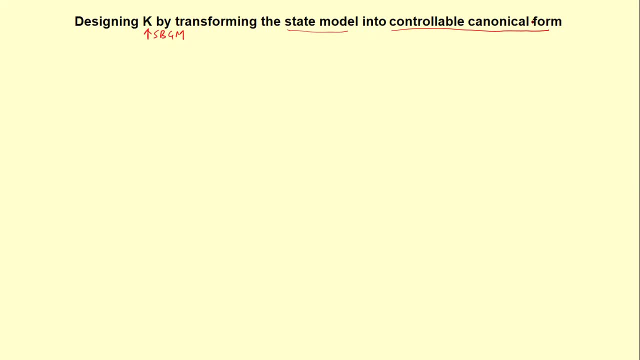 that our ab pair. it should be controllable. so we will first transform the state model, because every transform the state model to some controllable canonical form, and then we will obtain the state feedback gain matrix. right now, the characteristic polynomial of the given system is given by 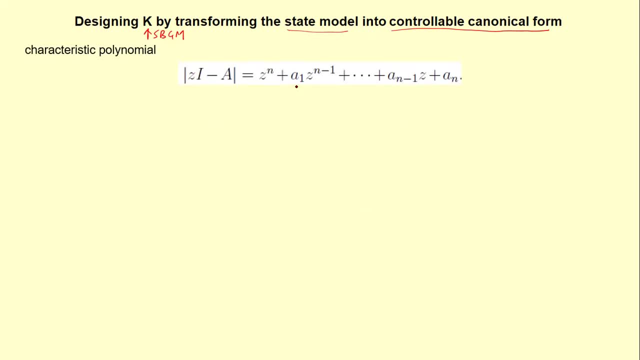 this equation, this is the characteristic polynomial, wherein a1, a2, a3, all these are the coefficients of z right, and this is your state matrix. this is the state matrix right now. if we take some controllability matrix now, controllability matrix, you see, is: 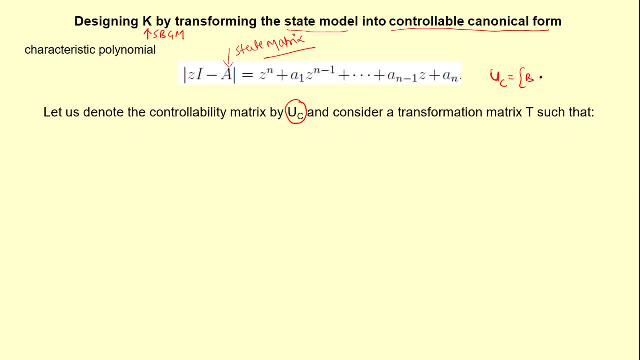 given by. as we all know, it is given by b, then a, b, then a square b. dot dot, dot, dot dot a and minus one b. so this is the controllability matrix for a given system. to be controllable, this, this matrix, should have full rank. the rank of this matrix should be full, that is N So. 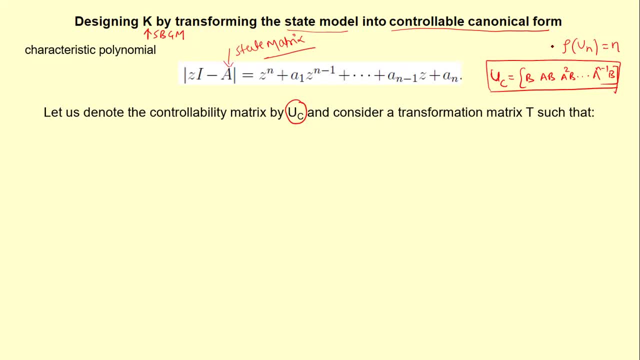 it should be the order of the system Now. first of all, we will take a controllability matrix. we will consider a transformational matrix, T, and this transformational matrix is given by the equation UC into W, where W is a weight matrix. this is the weight matrix. 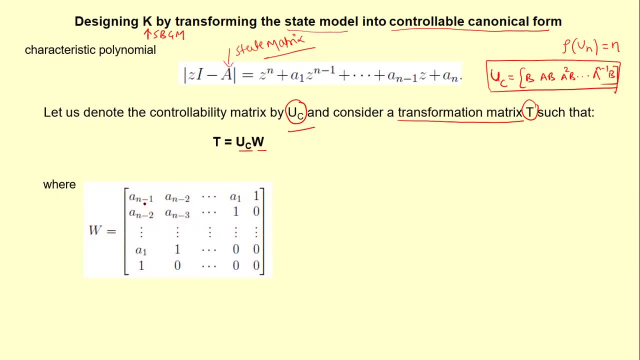 which is given by this equation. So we have all these coefficients of Z. So you can see, here we have the coefficients of the characteristic polynomial here. So all these ai's means, all these coefficients are the coefficients of the characteristic polynomial, All these. 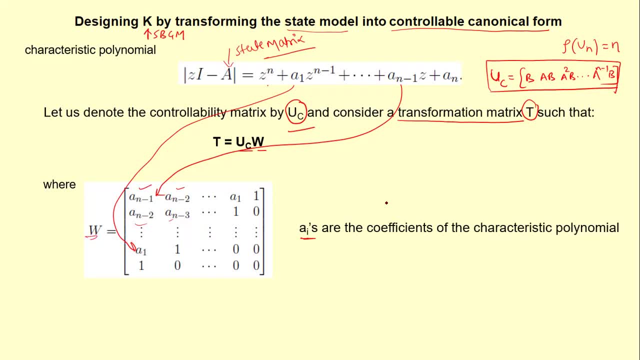 elements of matrix W. the weight matrix are the coefficients of the characteristic polynomial. Now, let us assume a new state. now, let us assume a new state, and this new state is this new state vector? sorry, a new state vector is X bar, such that it is related with the 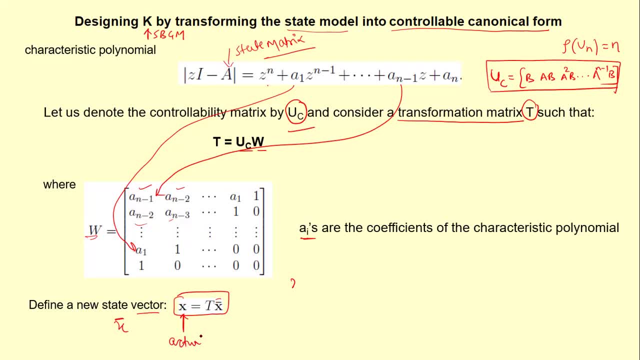 actual state vector. This is the actual state vector and this is the assumed state vector right. So we have used the transformation matrix, So we have used the transformation matrix So we can say that that X bar is equal to T inverse X, right. So this X bar, 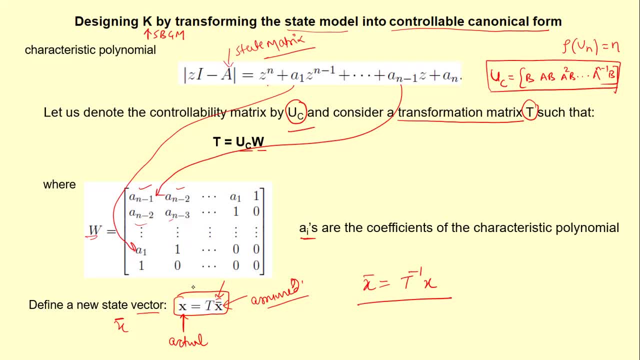 is the controllable form, controllable state vector, you can say So. we are using the transformation matrix to transform the actual state vector to the controllable form and hence this will given system by equation one, and equation one is x k plus one is equal to a x k plus. 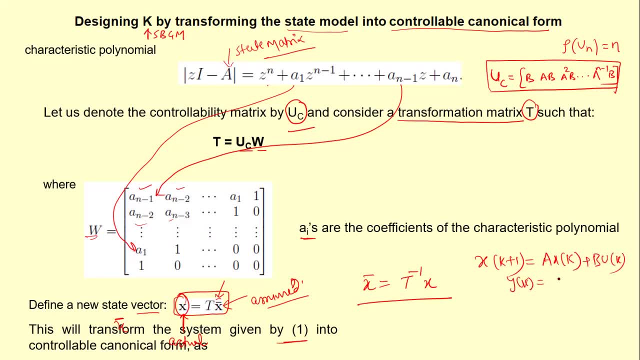 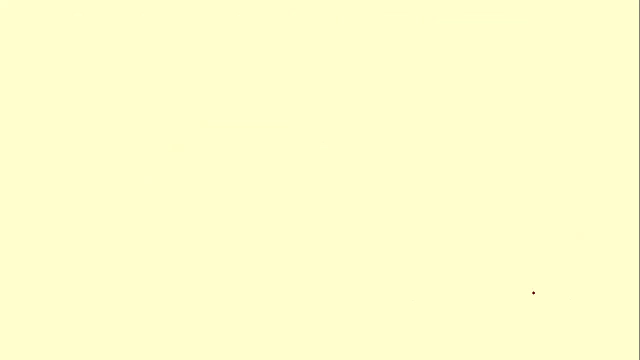 b, u, k and y. k is equal to c, x, k, right? so this will be transformed to controllable canonical form, right, and the new state equation will be: this is a new state equation, right, which is uh controllable, right? so that means this pair, a bar and b bar. okay, this pair is uh controllable, right? this is controllable now. 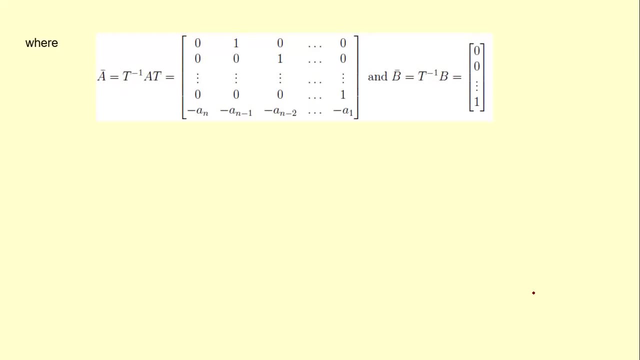 uh, this a bar and b bar are given by these equations, right? because, uh, uh, these are the controllable. uh, you know matrices, so our actual matrices will also be, you know, controllable. this pair will also be controllable right now. uh, let us find out. okay, so now, if, uh, we find out, 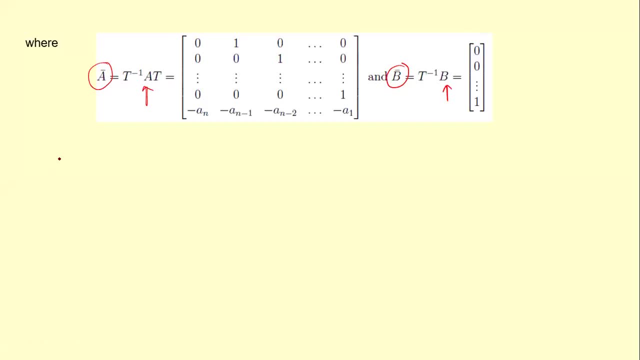 uh, this pair, a bar and b bar- is: uh, this is uh controllable, right? this is uh controllable, right. so we have a new state model which is x? k plus one uh bar is equal to a bar, x bar, k and plus b bar, u k. so we have a new state model here, right? and this pair, a bar and b bar, is. 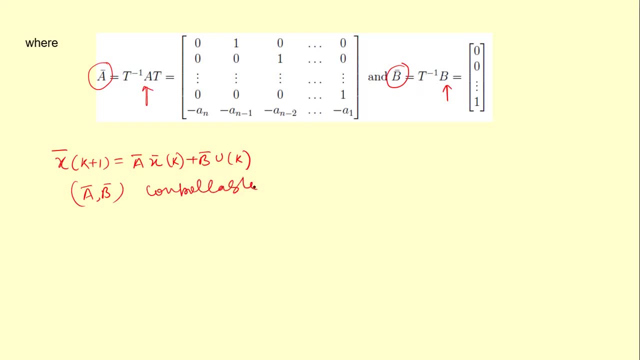 uh, controllable pair. so now, uh, we will first find out. so let us assume a new state feedback gain matrix k bar right. so, uh, now, such that the, such that the control law is uk, is equal to minus k bar x bar k right. this is a new control law, right? 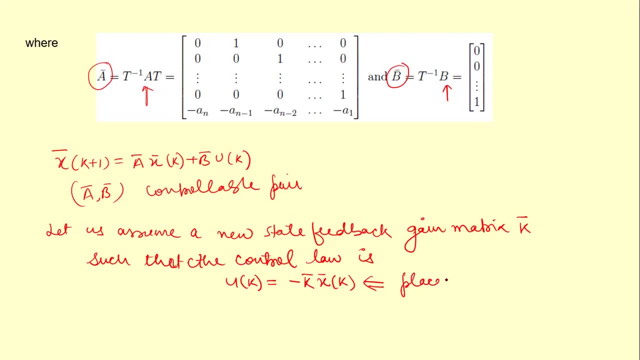 and this control law places the closed loop poles to the desired location right. that means this control law is also capable of placing the uh closed loop poles on the desired location right now. here this k is equal to. it is equal to k1, bar, comma, k, 2, bar, dot, dot, dot, similarly up till k and bar. so these are the elements of this matrix. 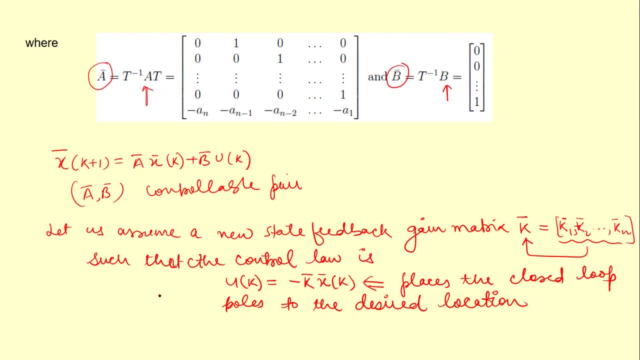 k right now because, uh, because x bar is equal to t inverse x, because we assume the new state k, which ma surely means that matrix. so now, if you enter the new state kingdom in a group here, okay, we assume the new state here, this one. so from this we can get: x bar is equal to t inverse. 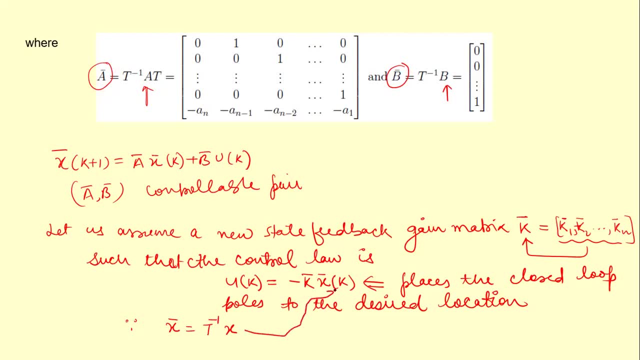 x. so we, we will put it here right. so uk will now be minus k inverse, sorry, k bar t inverse right and xk right. so now this control law. this is also control law, right? this is now updated control law. now, this control law will also place the poles of the original system, this control law. 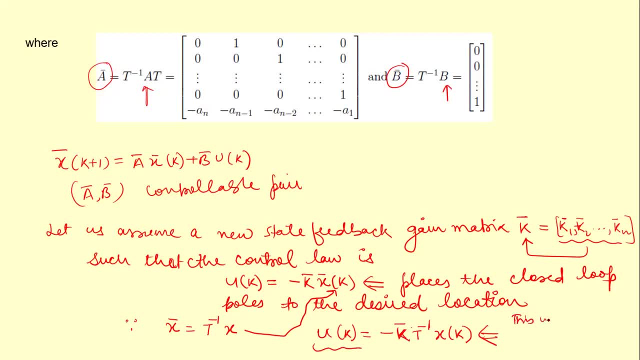 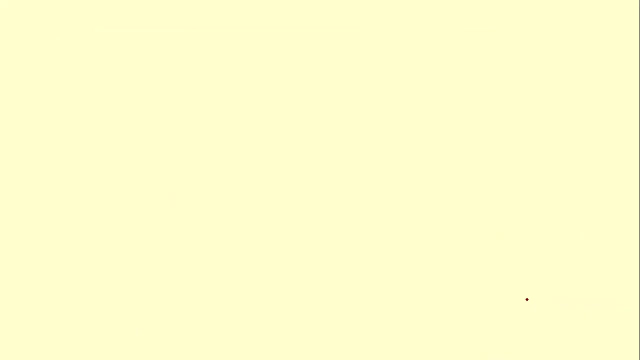 will also place the, the closed loop poles of the original system, right original system, to the desired location, right to the desired location. okay, so, uh now. so, if, uh, we place, if we see that, uh, all the poles and the given poles, uh, uh, the desired pole, these 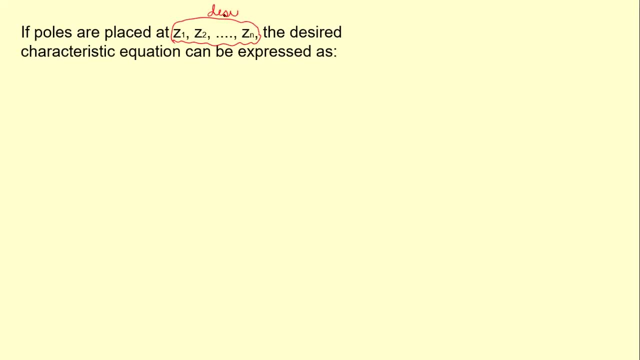 are the, let us say, uh, desired poles, right, okay, these are the desired poles. okay, so these desired poles will give us a desired equation, characteristic equation, and that characteristic equation is given here, so we can simplify this characteristic equation to get this one. this is, let us say, some equation number four. right now, 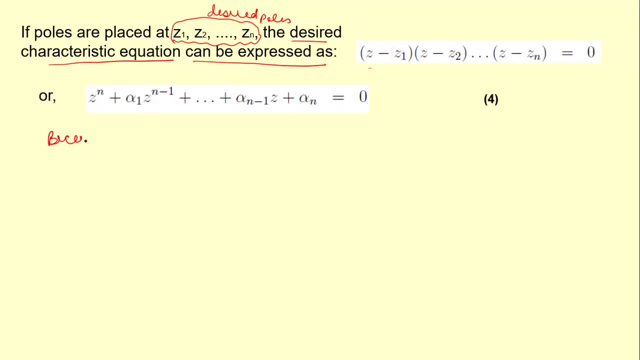 because your, uh, your pair, a bar and b bar, these, these two matrices, they are in controllable companion form, companion form. so, uh, we have this matrix here, right, so we can get this matrix. so we want that this k, this k bar should place the. the closed loop holds off a minus b bar, k bar in the. 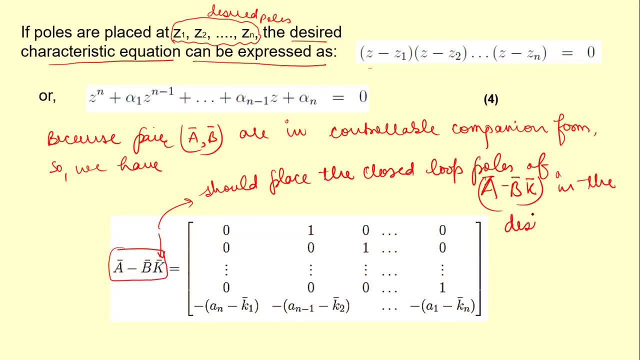 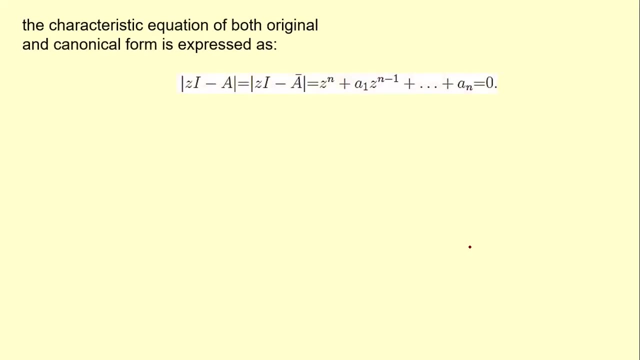 desired location. right, okay, so, uh, now let us uh see the characteristic equation of the original and canonical form. so, if we see the characteristic equation of original, this is the characteristic equation of the original system and this is the characteristic- uh, you know- equation for the uh canonical form. right, so if we solve this, we will get this one right now, uh, the characteristic. 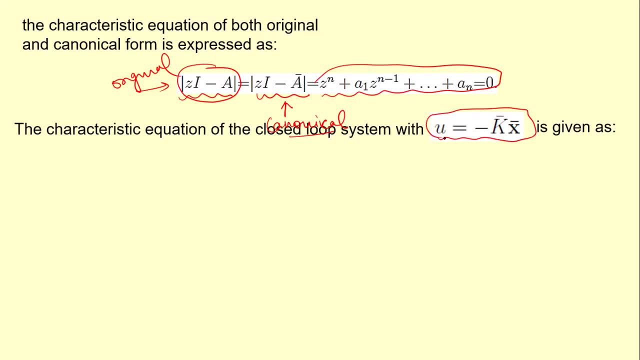 equation of the closed loop system with: if we put, take this as the control, or low, the characteristic equation will be given by this equation here. right, so uh, if we substitute, okay, so uh, this, this can be obtained by, you know, taking uh, the a bar minus b bar, k bar matrix. so 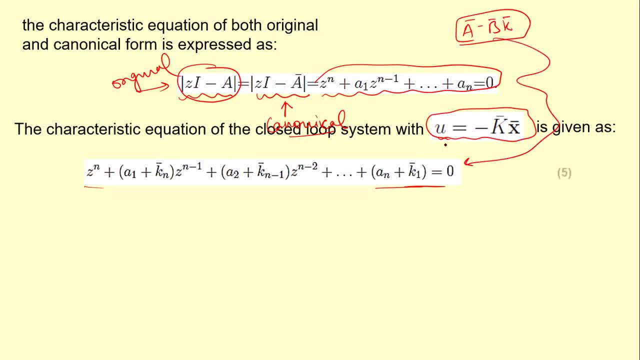 we'll take this matrix and we'll get this equation here right now. this is, let us, equation number five. if we compare this equation four and five, so if we compare these two equations, four and five, so equation number four is given on the last slide. this is the equation number four here. 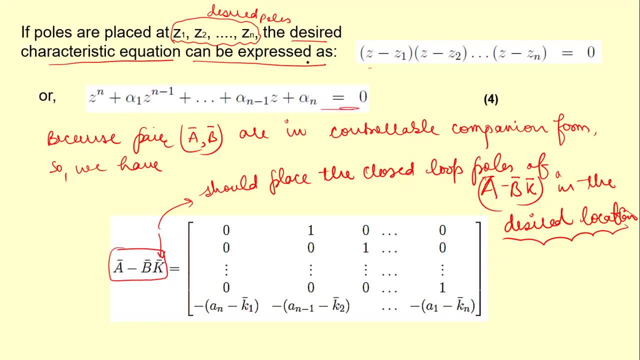 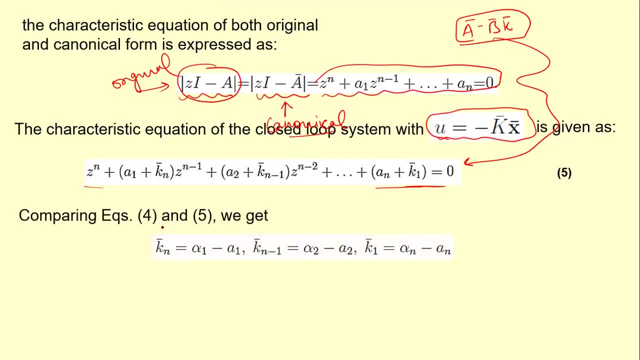 so here we have, this is the desired characteristic equation z, n, alpha one and all that right. so if we compare uh equation five with equation four, so we will get uh, the values of all these elements of matrix k, and this is, for example, some equation six. so that means 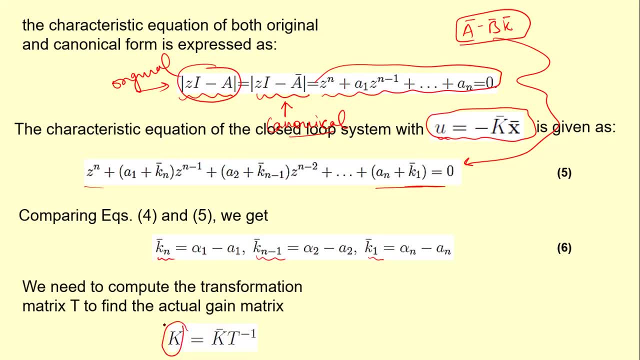 to get the state feedback gain matrix, the actual state feedback gain matrix, we need to find out the transformation matrix t and then we can multiply its inverse with the companion form gain matrix and we will get this k right. so there are the steps. if we have to, you know, uh, you know. summarize: 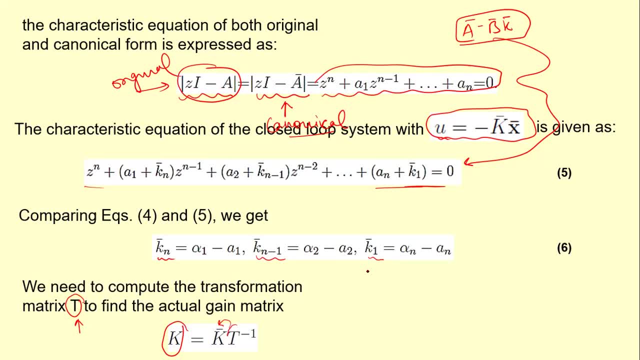 the whole, in theory, whole concept in some steps. so first step here is that, uh, obtain uc and uc is the controllability matrix. then the second step you can say is we have to check the open loop. characteristic equation, which is z, i minus a is equal to zero. this is the open loop. 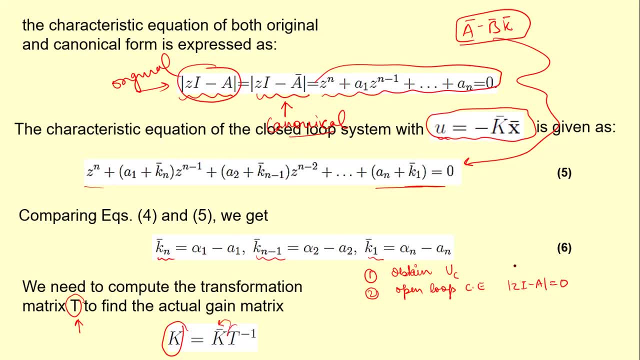 characteristic equation, right then. after that, we have to check for the desired characteristic equation and we have to check for the desired characteristic equation and we have to check for the desired characteristic equation and we have to check for the desired characteristic equation. right? so we have to check for the desired characteristic equation, right? so we have. 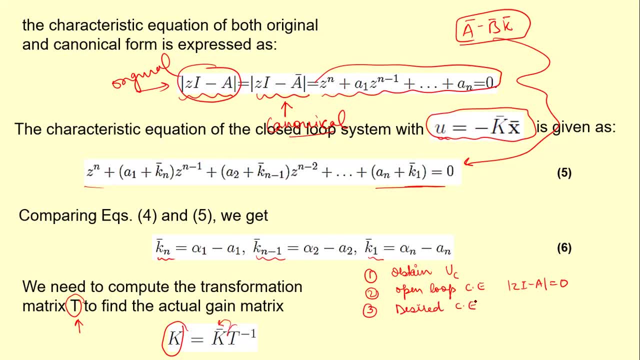 to check for the desired characteristic equation. right, so we have to see the desired characteristic to see the desired characteristic equation. uh, so desired characteristic equation is z minus uh, so desired characteristic equation is z minus uh, so desired characteristic equation is z minus z1, z minus z2, dot, dot, dot, z minus z n is equal to. 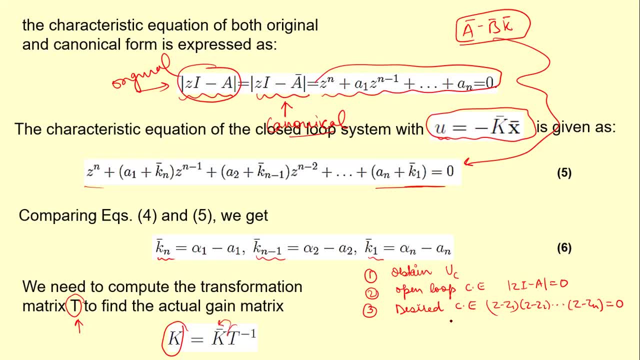 z1 z2 dot dot dot z minus z n is equal to z1 z2 dot dot dot z minus z n is equal to zero. so this is the desired characteristic equation zero. so this is the desired characteristic equation zero. so this is the desired characteristic equation. and then finally, uh, we have to. 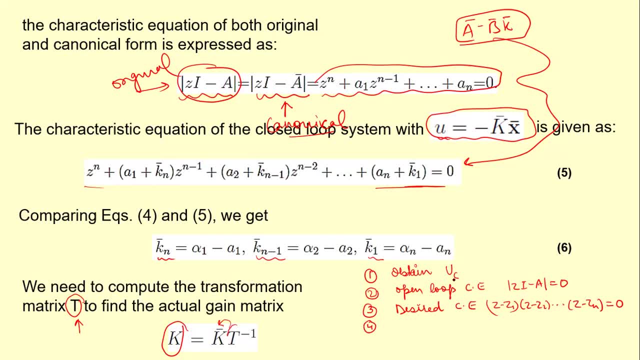 and then finally, uh, we have to. and then finally, uh, we have to. um, you know so, here we have to obtain uc. um, you know, so here we have to obtain uc, we have to obtain w. uh, w can be obtained here. so we'll write open loop characteristic equation and: